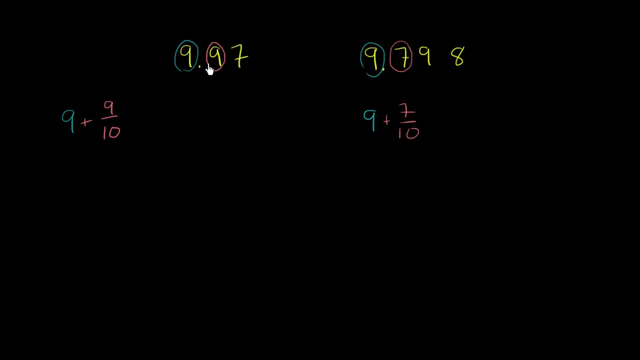 And this is at 9.9.. So you can really just look at the discrepancy in the largest place value to recognize which number is greater. This has 9 tenths. This has 7 tenths. It doesn't matter what's going on in the hundredths. 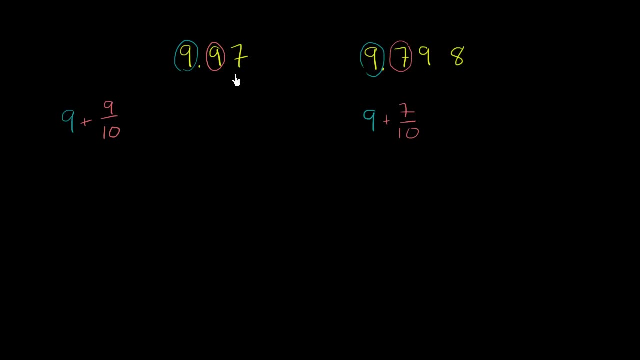 and the thousandths place. And, to make that clear, let's actually add up these numbers and compare them as fractions. So let's keep on going with this. So you have 7 hundredths here. So you have 7 hundredths here. 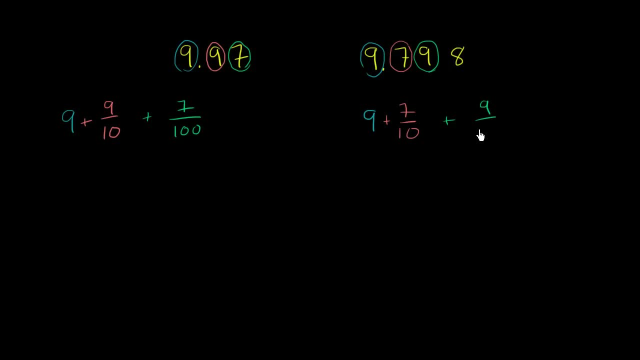 And here you have 9 hundredths. So here you have 9 hundredths. And then, finally, here you have 0 thousandths- And here let me do that in a different color- I already used blue- And here you have 8 thousandths. 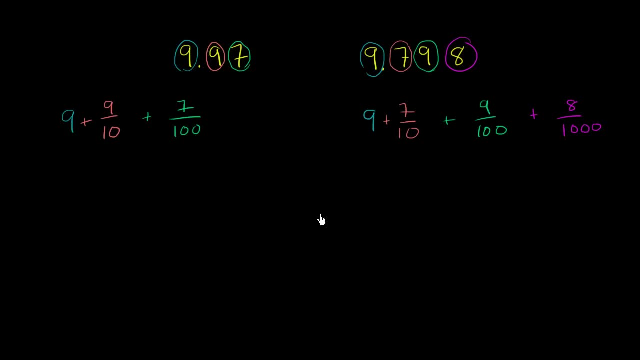 So plus 8 over 1,000.. So let's put everything in terms of thousandths so that we can add these all up and have two fractions over thousandths or things in terms of thousandths. So 9 is the same thing as 9,000 over 1,000.. 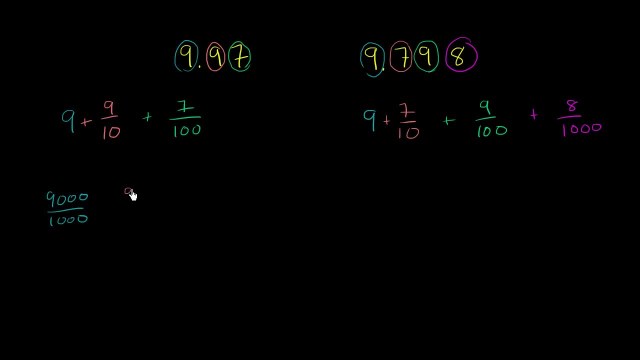 9 tenths. well, let's see. If you multiply it by 10, you'd get 90 over 100.. Multiply by 10 again, you get 9 hundred thousandths. 7 hundredths multiplied by 10 is 70 thousandths. 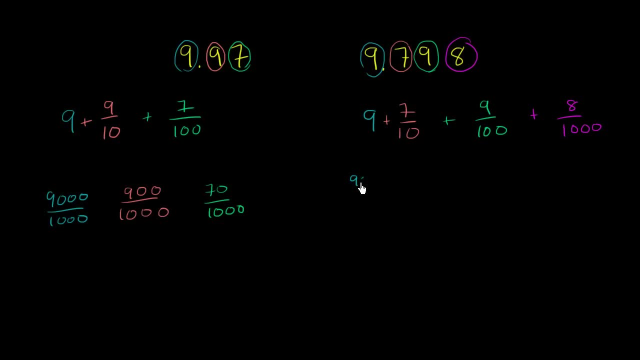 And let's do that over here Once again: 9 is 9,000 over 1,000.. And then plus 700 over 1,000.. Plus 90 over 1,000.. Just multiply the numerator and denominator by 10.. 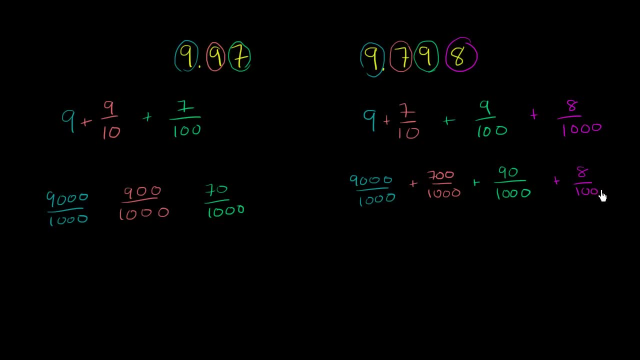 Plus 8 over 1,000.. And so what is this number on the left? This number on the left Is: how many thousandths is it? It's 9,970.. So it's 9,970 and 70 thousandths. 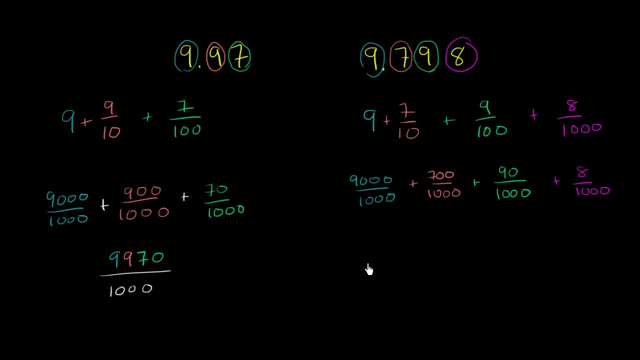 While this number on the right here is 9,970.. So this number on the right here is 9,970 and 70 thousandths. So this number on the right here is 9,970 and 70 thousandths. So this number on the right here is 9,970 and 70 thousandths.